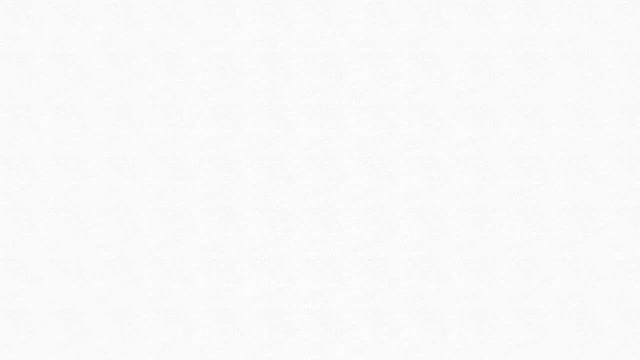 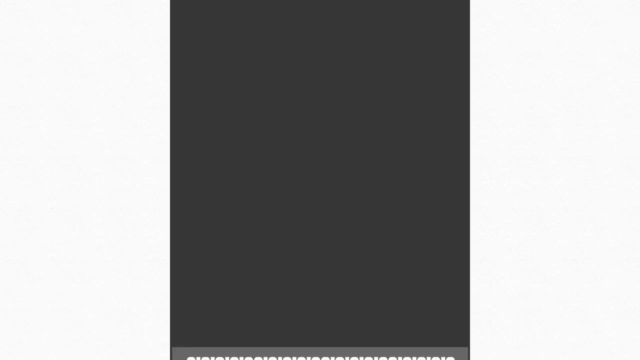 are carried out. Do not always be fooled, though. The efficiency of the processor's architecture determines how much work the processor actually does. The bandwidth determines how much information can be processed in one instruction. The wider the bandwidth, the more that can be fitted on and sent. Think of it as a motorway. The 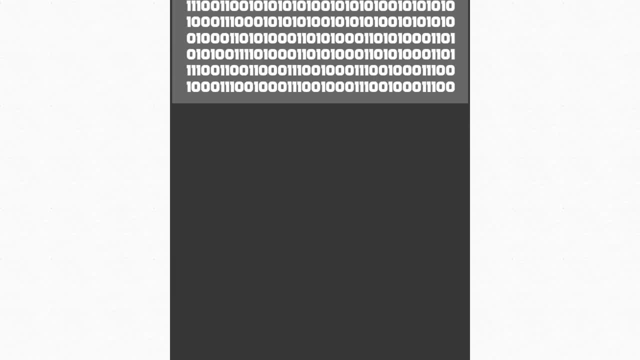 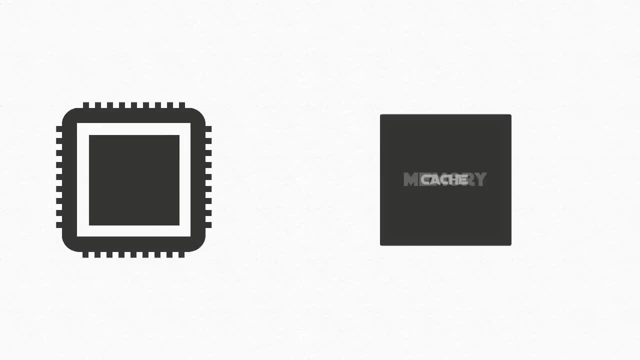 wider the road, the more cars- or, in this case, instructions- can be run at the same time, The processor has its own version of memory, also known as cache. that exists on the die of a processor Because it has less time to travel. 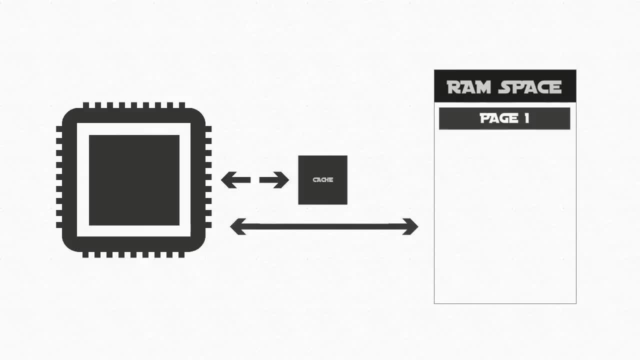 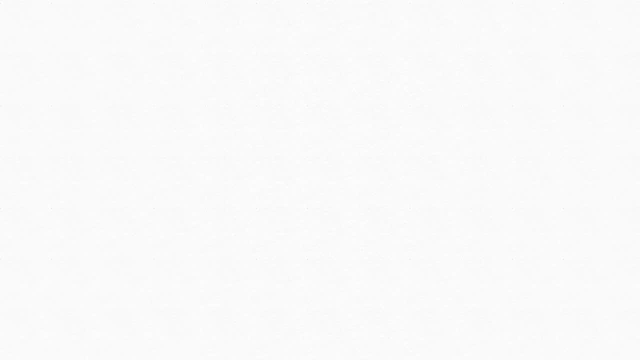 it is usually checked first before calling in. a page from the RAM Cache can be accessed between five to ten times faster than accessing the RAM. A process scheduler is in charge of making efficient use of the physical processor. There are two parts to this. One is the job scheduler. 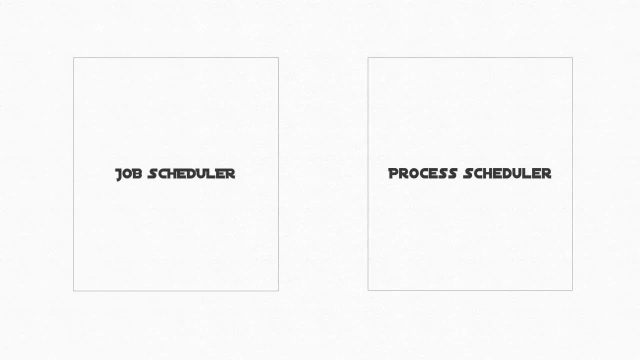 and the other is the processor. The processor is the job scheduler and the other is the processor- process scheduler. taking note that a job can consist of many processes. It can juggle many jobs. A process can be in five different states: Hold ready, run, wait and finish. Hold is: 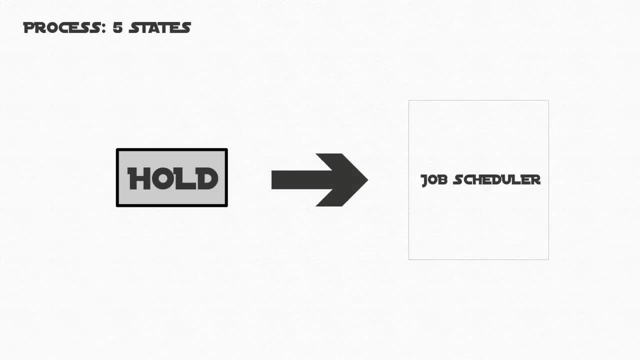 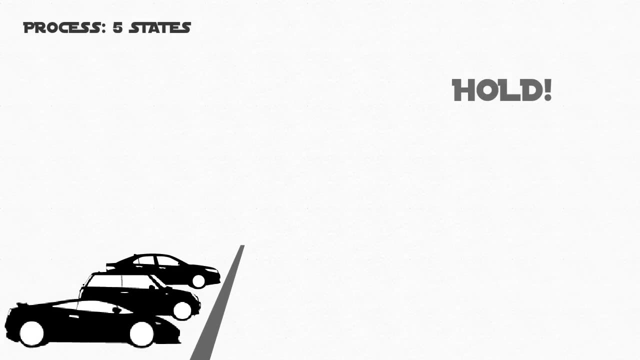 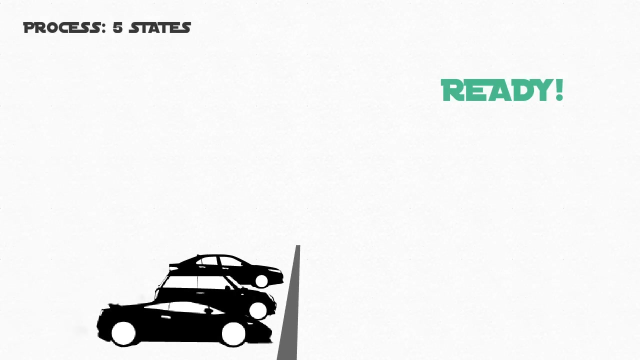 controlled by the job scheduler and, as the name suggests, it is holding the job until it has permission to run. Think of a car race. You cannot start the engine until the starting signal has been called. Now, when your engine is on, you are in a ready state. The ready. 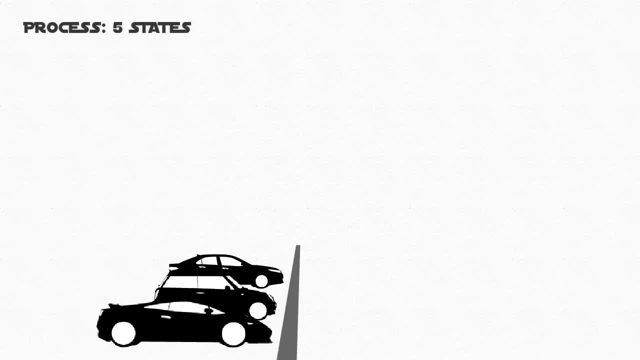 state is a signal to continue with the process. When the car is ready to proceed, it is in a running state. In our case, it is currently processing the job. Throughout this time of running, there may be a concern of performance, So a check with the team is made to ensure it. 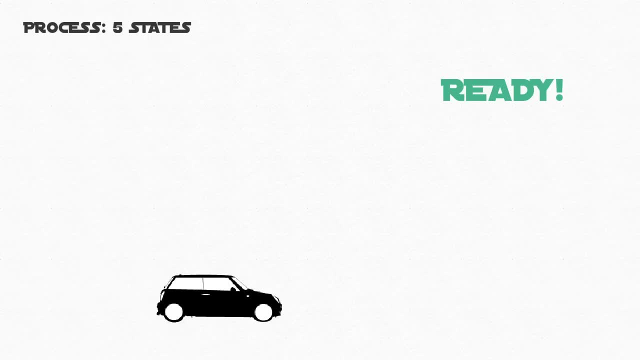 is okay to start running again, returning to a ready state. If it is okay to run again, it goes back into a running state. But what if there is an engine failure? In that case, an IO request page fault is presented and the car is put in a waiting state.